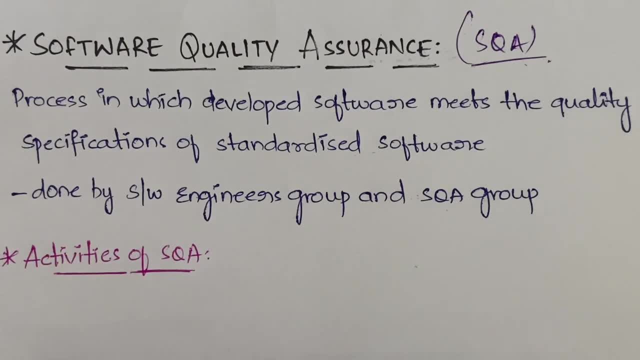 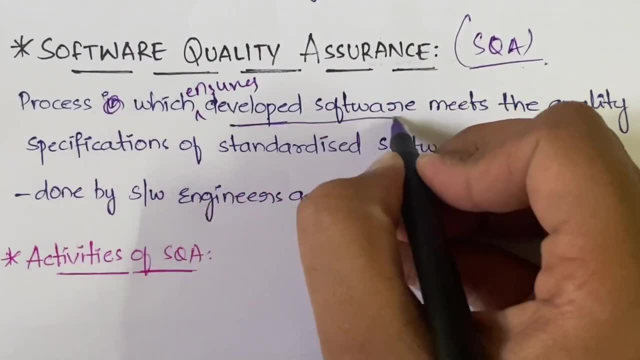 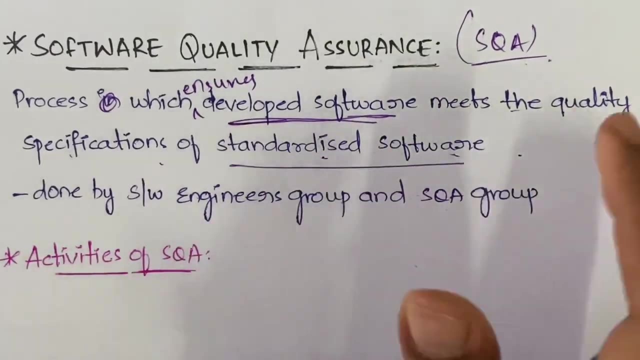 The name itself says so. it is a process in which it is a process in which, instead of this we can like, which ensures that the developed software meets the quality specifications of the standardized software. See Developed software, standardized software right. Standardized software is nothing but the already. 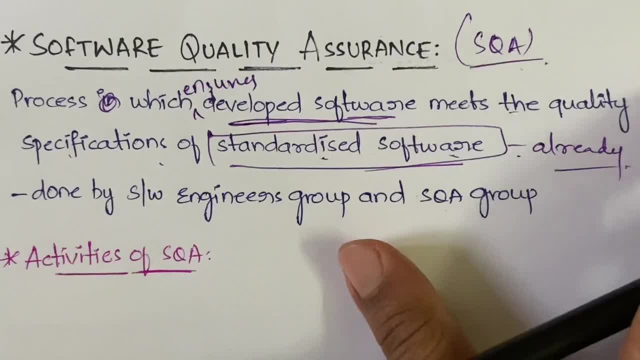 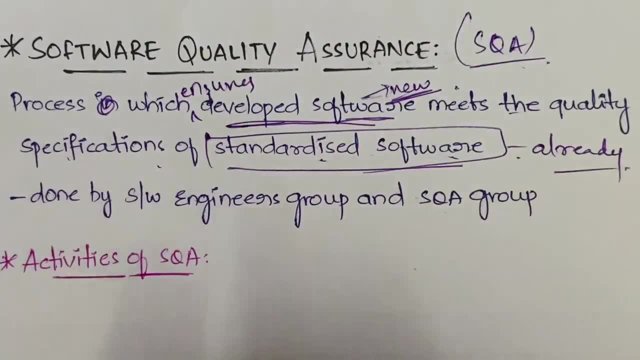 existing software. Okay, the software which is already existing, Developed software, is nothing but the software which we have developed newly Got it. So, in software quality assurance, what we will do is whatever the standards are there. what existing software standards are there, right? So? 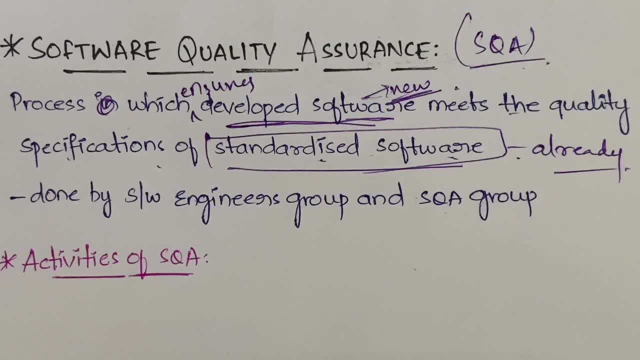 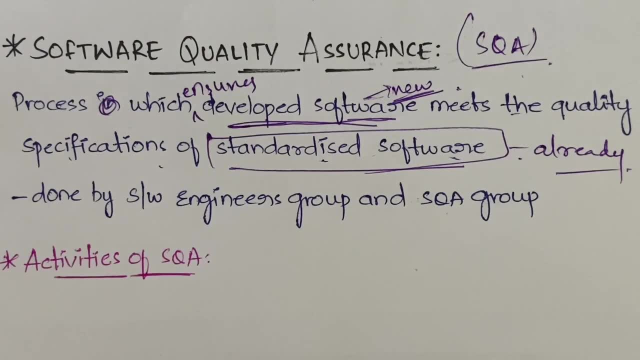 it will ensure that whether the software which we have created newly will meet the quality requirements, That is, is on par with the in terms of quality with the existing standard software, or not. Okay, see, suppose when you're drawing something you will be having a model in front of you right, You're drawing a. 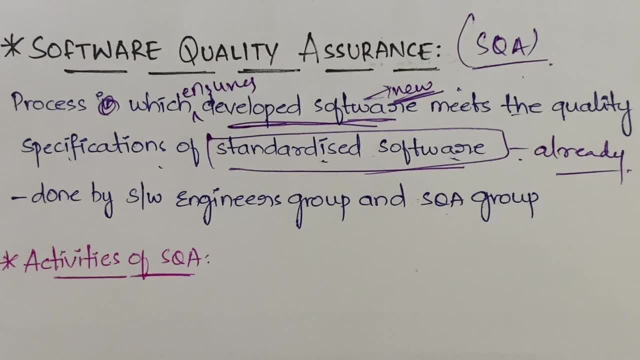 picture of a waterfall or a mountain or whatever it is. you're looking at it and you're drawing. then, after you complete your sketch, what you will check? whether your picture is according to the original picture or not. Here also the same thing: you will already have a standardized 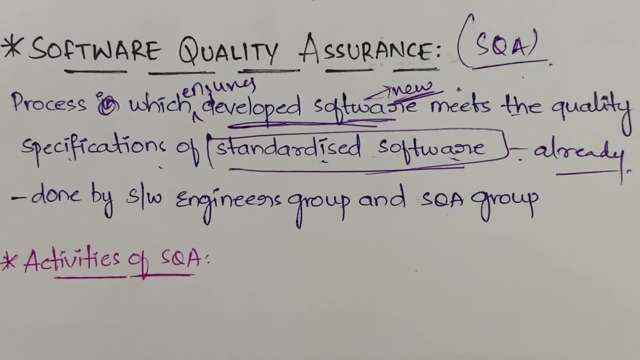 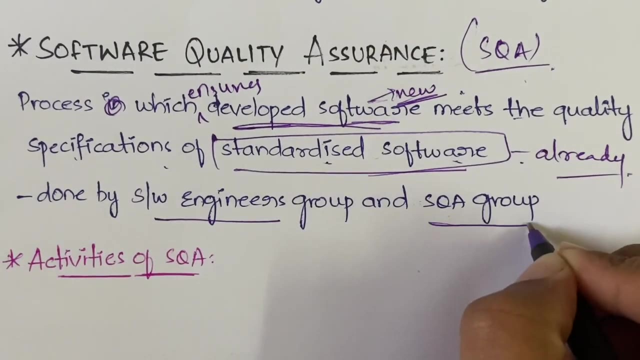 software. quality requirements, quality standards, right. So whatever software you have created newly, whether that is according to the standards of the existing old one or not, that is what you will check in this. very simple: It is done by the software engineers group and the SQA group. Okay, so software. 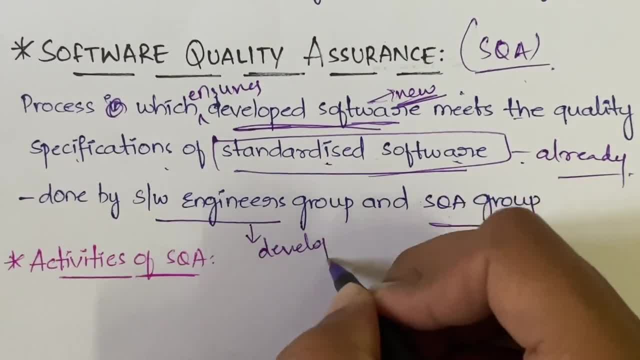 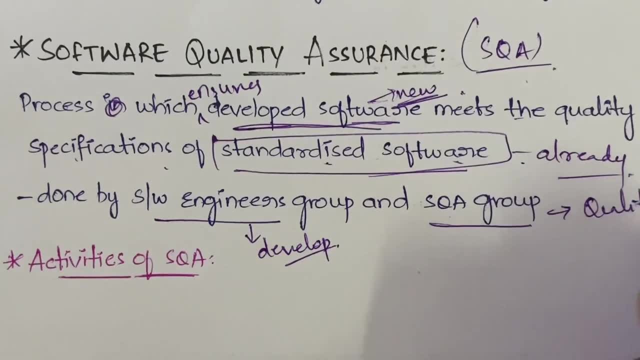 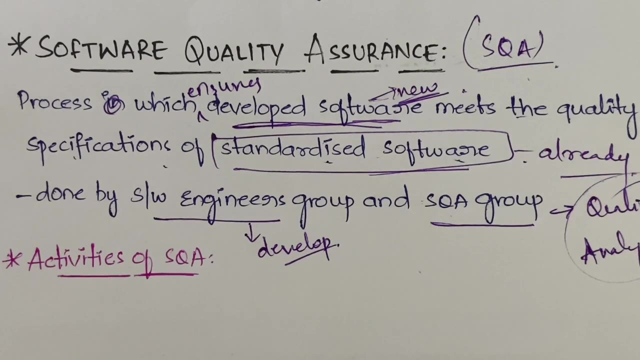 engineers. they. what they will do is they will develop the product. they will develop the product and SQA group. what SQA group will do is they will be performing quality assurance And quality assurance analysis. some quality related tasks they will be doing. Okay, so it is done by the combo of both software. 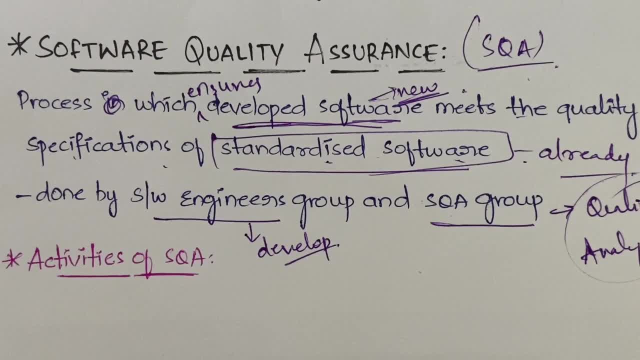 engineers and the SQA group. both together they will do a. software engineers are concerned about development and SQA group is concerned about the quality analysis of quality. you know, reporting, assurance and all Got it. And now let us see what are the activities of SQA. So actually we have activities of SQA. that is what all have to be performed in. 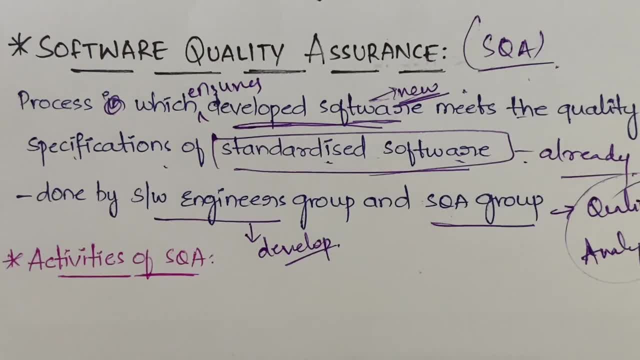 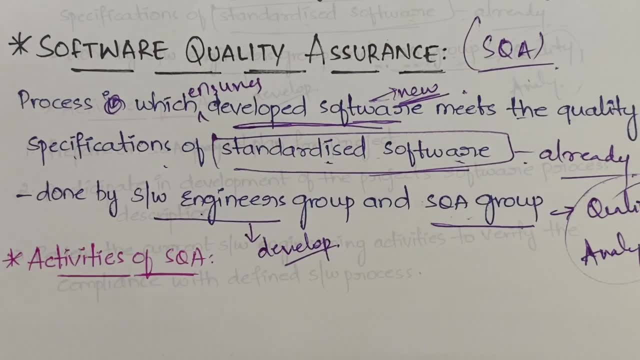 order to establish the software quality assurance. So all these activities which I'm going to tell you now are performed by these people only: software engineers and SQA group. Okay, by now we've got to know what is SQA. right now, let us see what are the activities of SQA. 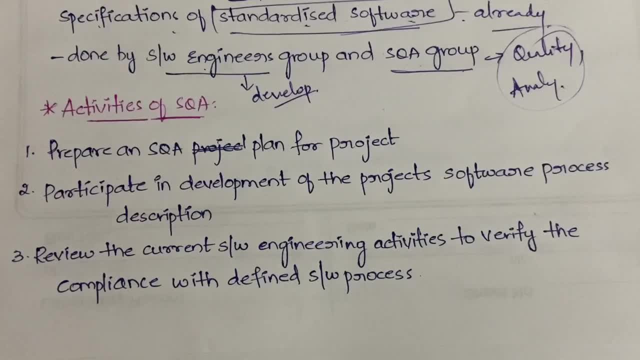 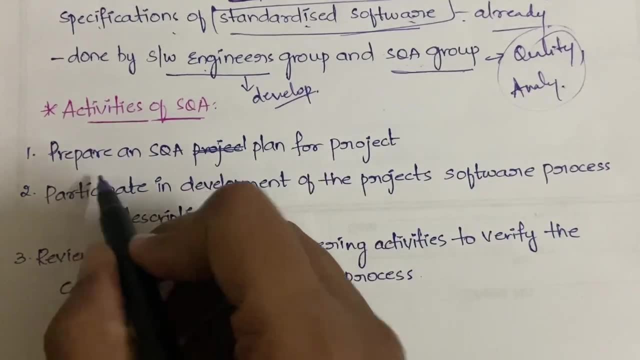 activities of SQA is nothing, but you can also say tasks: what are done in a software quality assurance right? First, what we have to do is we need to prepare a SQA plan for the project, not only for SQA in general, also, if you are starting any. 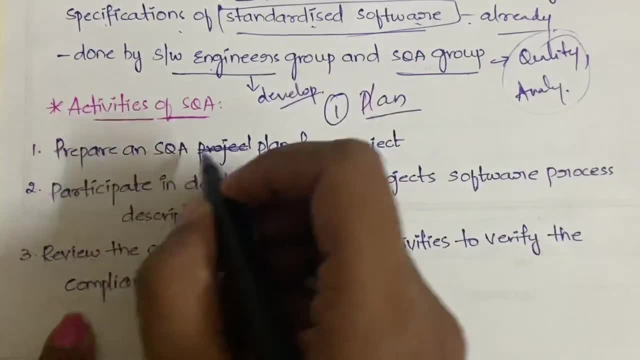 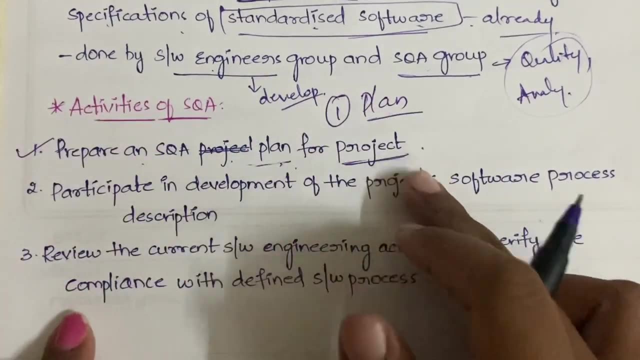 work. what is the first step that we do? we write a plan, right. So here also, in the first step, you need to prepare a SQA plan for the project which for which you wanted to perform the SQA. Okay, once you're done with SQA, second, what you have to do is you need to 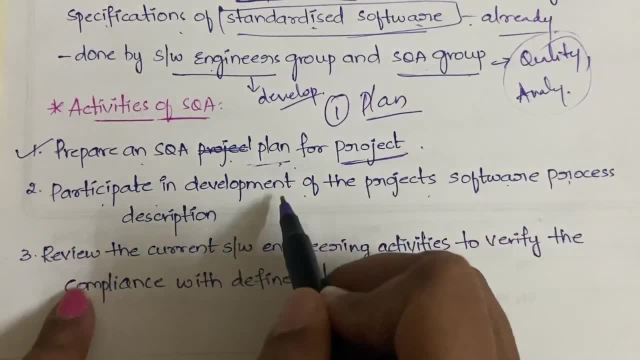 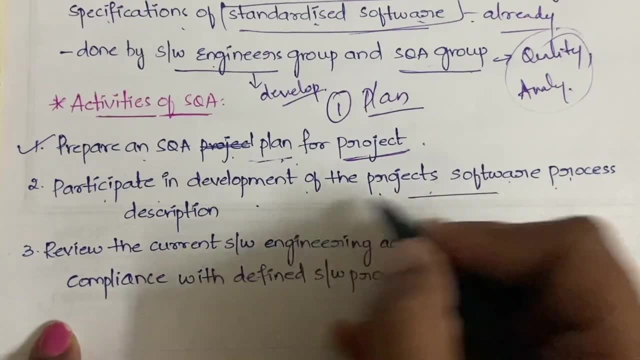 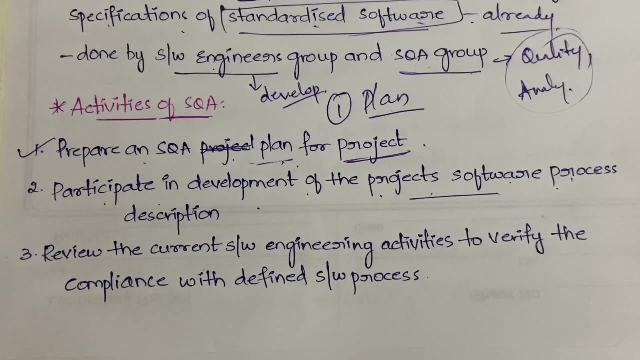 participate in the development of the project software process description, which is simple. you need to participate in the development of the project software process description. that is all the development of all the software related to the project. the project will have both hardware and software sites right, So whatever hard software is required for the project software. 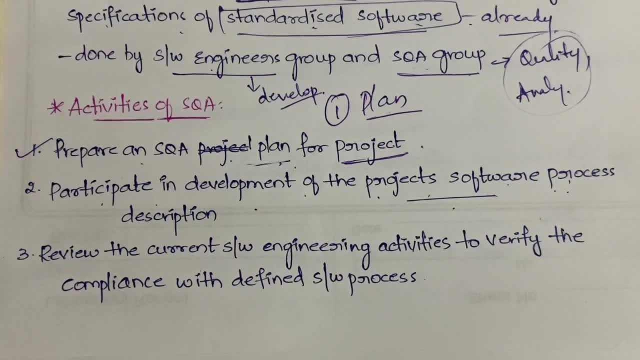 process description. so you have to go and participate in the software process description. that is when the software of the project is being defined. you need to participate there, you need to be there, you need to listen, you need to understand what is the software. 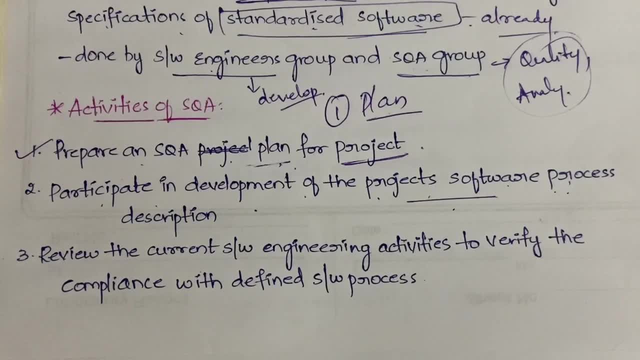 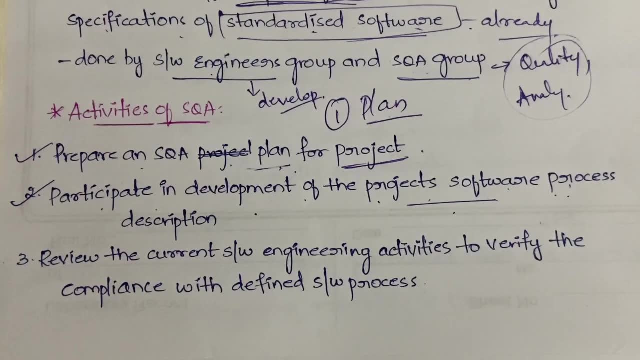 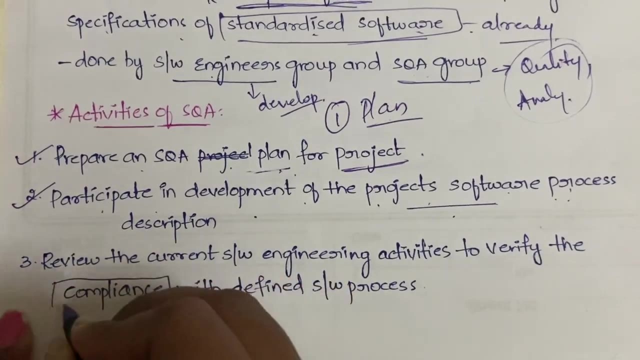 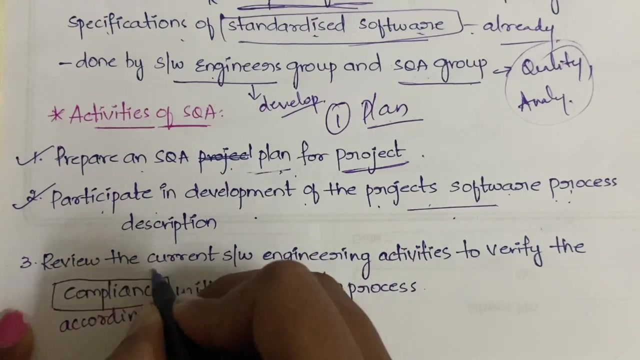 that is being used for the project Got it. Next, Review the current software engineering activities to verify the compliance with the defined software process. Very simple Here, in place of compliance, you can remember it as according to: Okay, so you have to remove. review the current, current in the sense the present, the. 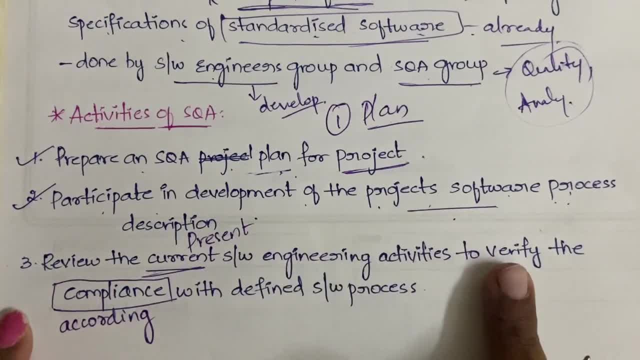 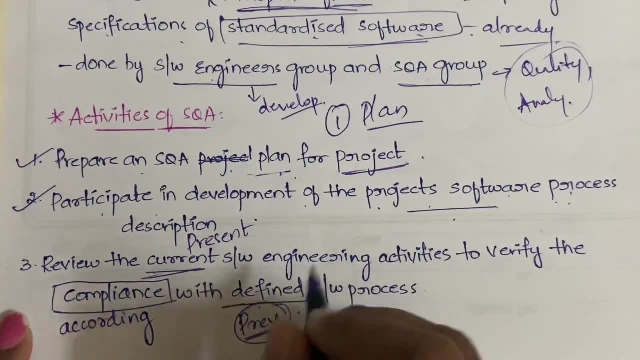 present software's engineering activities should be verified with the defined. defined is nothing, but you know previously already pre existing software is there, read. So whether both are matching or not. that is, we are matching the standards of the predefined software or not. So whatever software. 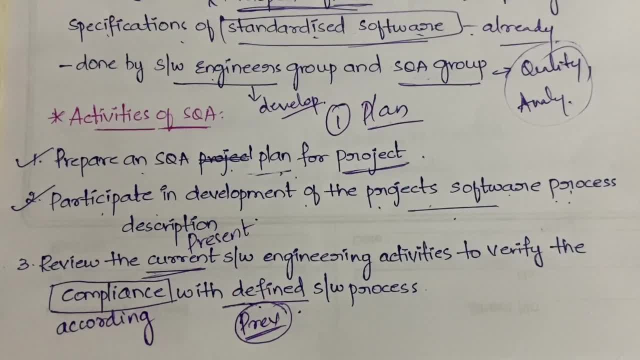 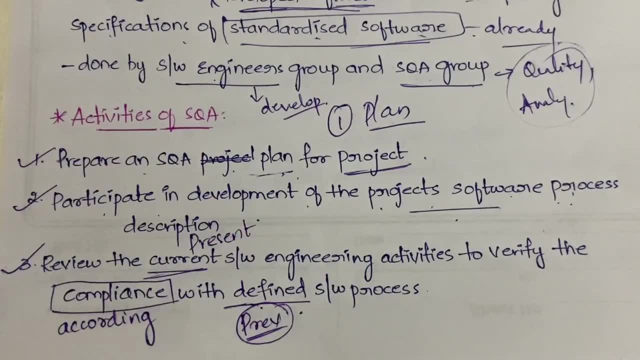 These are to be done. All of them are done or not, That is, we have to check, okay, Next. So, first time, what we're doing, we are preparing our plan. the second step What we are doing, we are participating in the software description, like: what is the software?